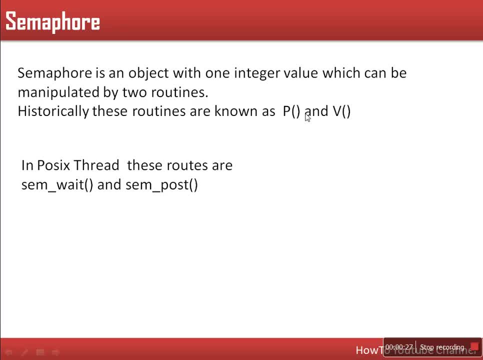 which is used for decreasing that value and V for increasing that value. So P sometimes we also call it weight and V also call it signal. In POSIX thread these P and V operation actually named as SEM underscore weight and SEM underscore force. So semaphore basically is an integer, is a variable, there is a value and this value can be accessed or can be manipulated by only two operations. 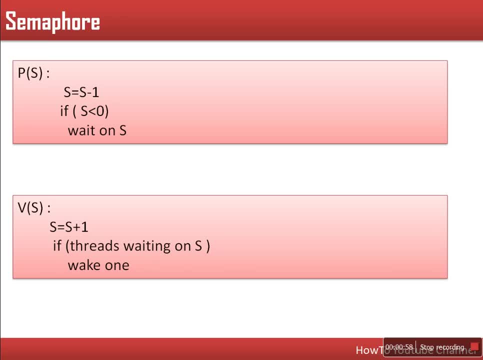 And these operations are atomic, Now, and so these are the definitions for operation P and V. So this operation P, what this operation will do? it will decrease the value of S And now, if this value is less than zero, it will keep on waiting. 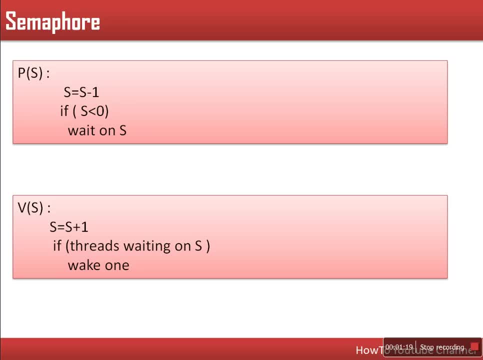 So how this waiting can be achieved, one way is that if there is a while loop with this condition, so that while loop keep on running, So that will be a busy waiting And this V operation, this V operation will increase the value of S. Now, if it will find that there are some threads which are waiting for this semaphore S, it will wake one of them. 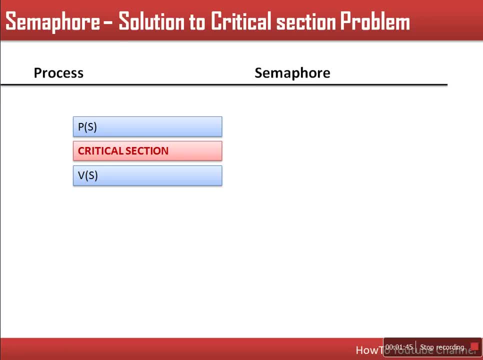 Now so how this critical section problem can be solved using semaphore. So what can be done before entering to the critical section? P operation will be called, And this operation will decrease the value. So let's take a semaphore and the value of S is initially one. 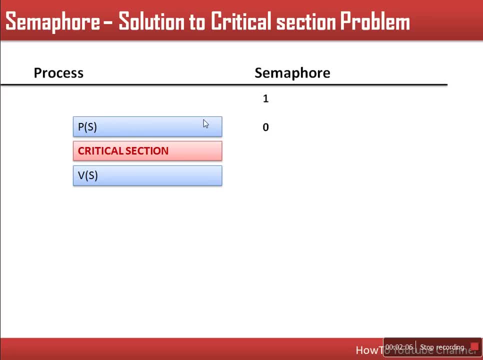 So when this operation is called, this operation will make it this value to zero And after making this value, this process start its critical section. At the end of critical section it will increase this value again by one. So in case if there are another process which also wants to enter in critical section, 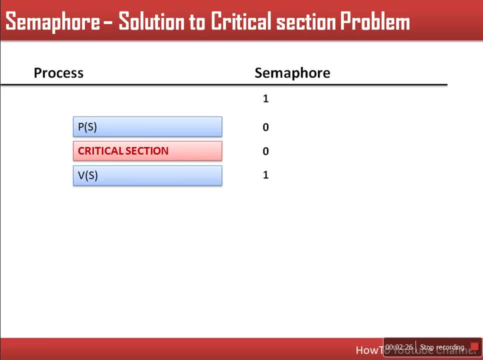 So that process also will be having the same code. So when that process call P, So that P actually decrease the value and it will make this value zero to minus one And that process actually keep on waiting. So we will see example, if we are having two process, how this mutual exclusion will be achieved. 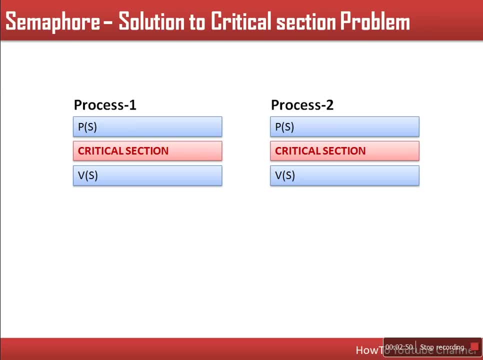 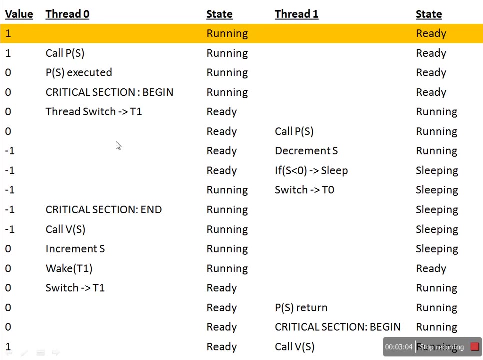 How it will solve the critical section problem. So these two process will be having same code. Now we will see the execution of these two process And for our example, actually we have taken thread, So we are considering same code for thread. So here it will show you the value of semaphore. 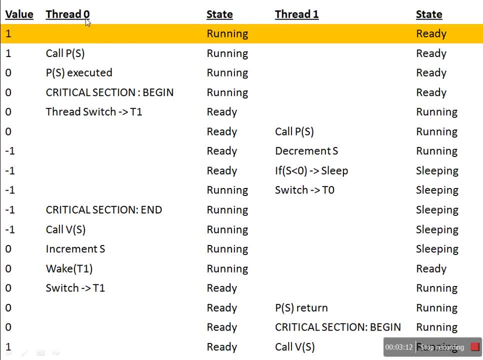 This will show you the thread, first thread, which is thread zero, And it will show which statement is executed Here. it will show the state of thread first thread And here- this is second thread- all code when these instruction will be executed And here, state of thread. 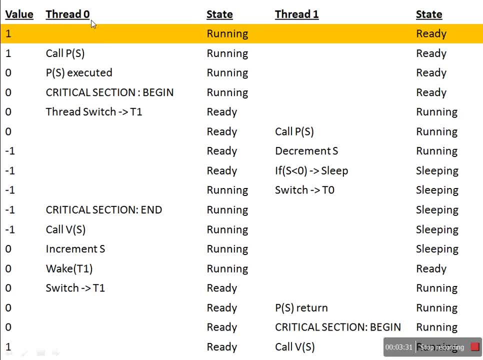 So here we are, assuming initially thread zero, start executing. So state of this thread is running And some other threads are also available there And those thread actually ready, they are waiting to run, They are waiting for CPU. So this thread is active, this thread is running. 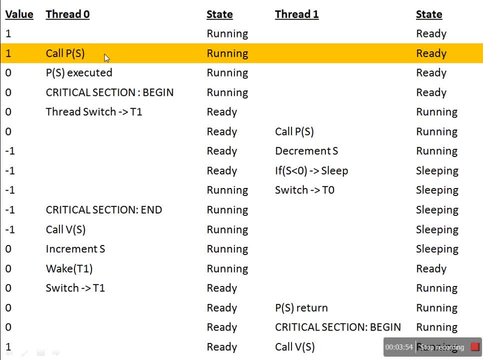 So this thread will call PS operation. So what this PS operation will do? it will decrease the value of thread. So here, when we call PS operation, value of semaphore is one, But when the execution is completed, this value become zero. Now this P operation says that if this value is less than zero, in that case wait, otherwise continue your execution. 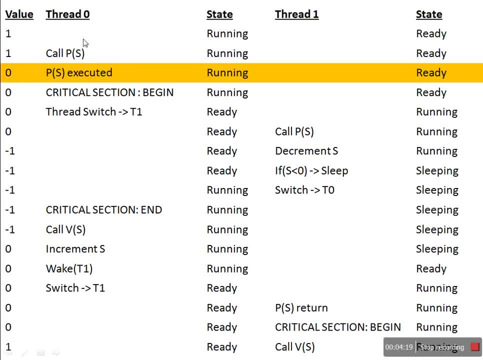 So this value is not less than zero. So this thread will keep on executing its instruction. it will come to the next instruction, So it will enter in its critical section. Now let's assume while executing its critical section there is a interrupt and operating system actually switched to another thread. 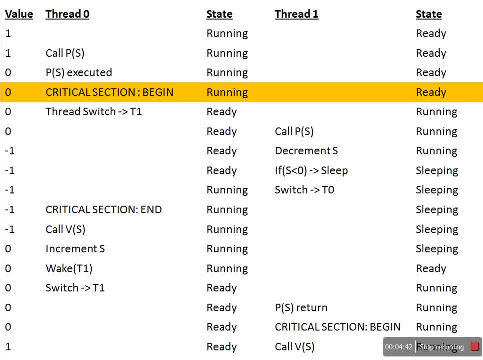 Our CPU actually start executing to the another thread. So how this scenario will be handled? so here we are, assuming there is an interrupt and CPU actually start executing another thread. So when this interrupt occur, first thread will change its state and it will come to the ready state, and second thread will come into running state. 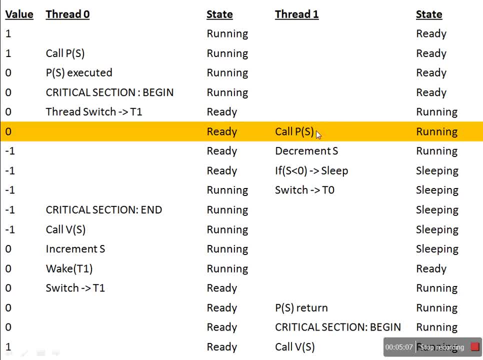 So thread second thread also will do the same code. it will execute the same code. it will call P operation. So this operation will decrease the semaphore value, which is currently zero. after decreasing it will be minus one, Now this operation also having this code. if this value is less than zero, then go to sleep mode. So here this condition is satisfied and this thread voluntarily release the CPU and it will go to the sleep mode. So its state is actually change to sleeping or waiting, And after sleeping this state CPU will be switched to first thread because this thread is voluntarily releasing the CPU. 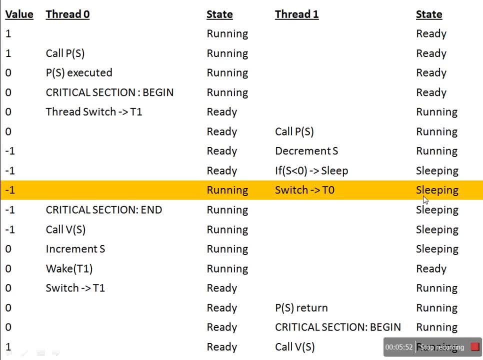 So when this switch occur, this thread- actually this thread- is in sleeping mode and first thread will start running. So here we are, assuming, let's say, critical section execution of first thread is done. So when critical section executed completely, this thread will call V operation and this operation will increase the value of S. 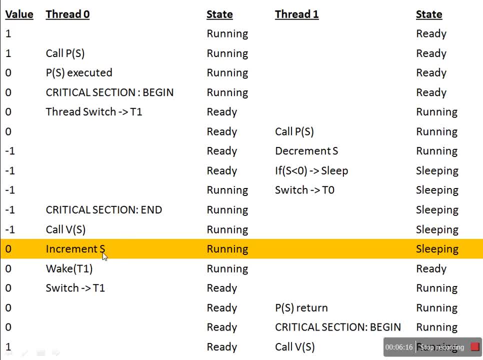 So this value become now zero. Now, if code of V operation says that increase the value plus, if there is any thread waiting, wake that thread. So here, if you can see, this second thread is actually waiting for the semaphore. its sleeping, So it will wake. second thread here. 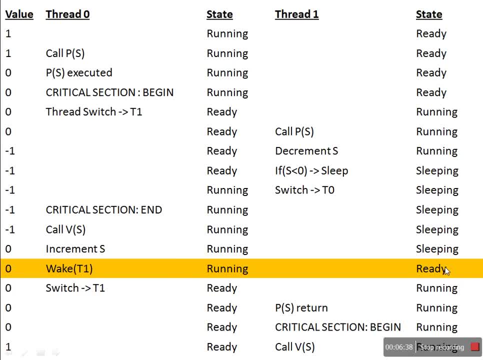 So now this thread will change its state and its now ready to execute. So here execution of thread. one is completed, first thread completed successfully. So when this execution of this thread is completed, CPU will switch to the another thread, So switching will occur here. 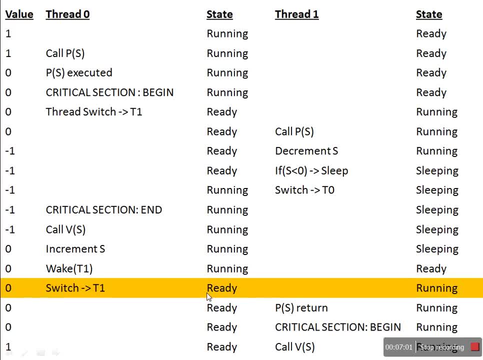 So after switching, this thread will change its state to ready- and we are assuming there are some other code as well- And CPU will come to second thread. So here it change its state to running Now. here this thread actually called P operation. here It decremented value. but it find that value negative one. that's why it go to the sleep mode. 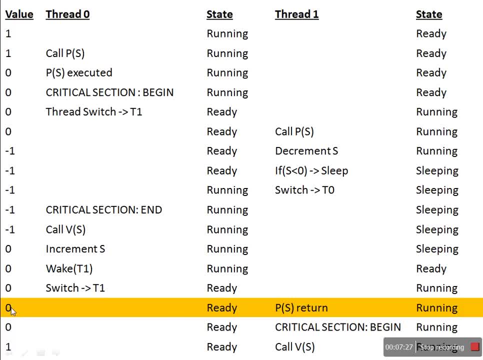 But here it sees the value. that value is zero and P operation says that if value is zero, then continue your execution. So second thread will continue its critical section And once this critical section is completed then it will call V operation. and this V operation actually increase the value of semaphore.